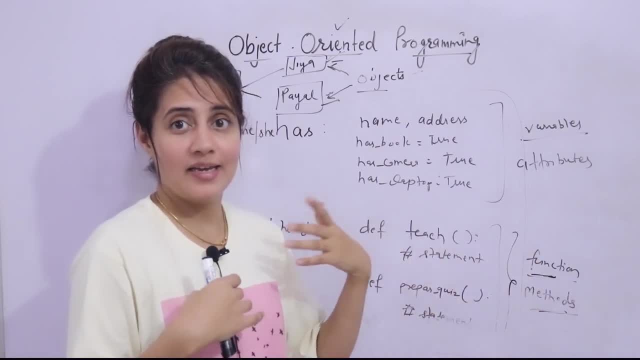 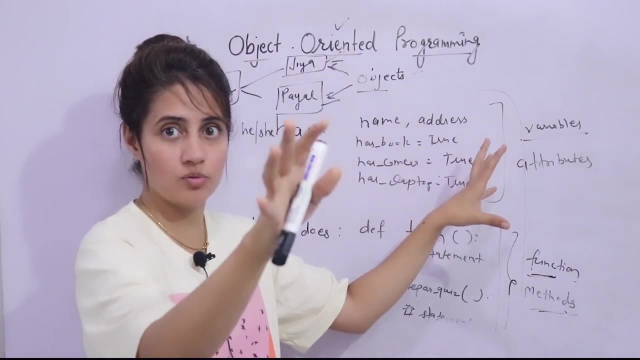 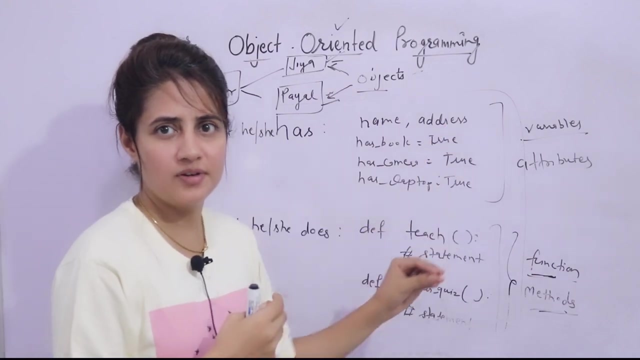 channel Right. So, like I was the manager and I have instructor, I have had instructor. then I have editor and social media marketer to handle their respective job Right Now I have hired like two instructor, Jenny and Jia, to teach different, different subject right. So these were objects and the 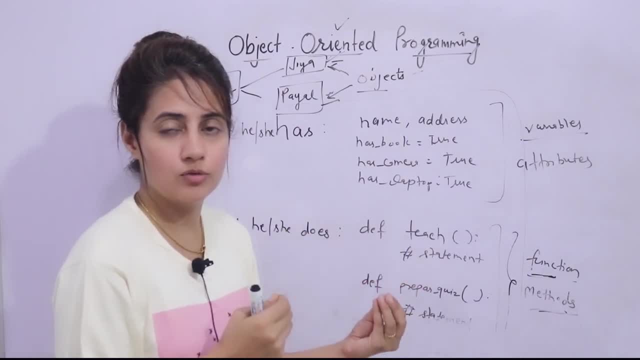 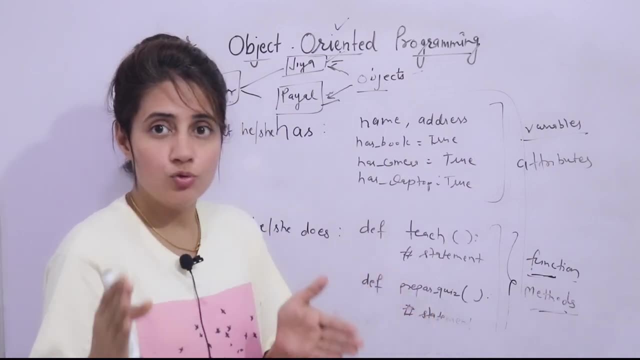 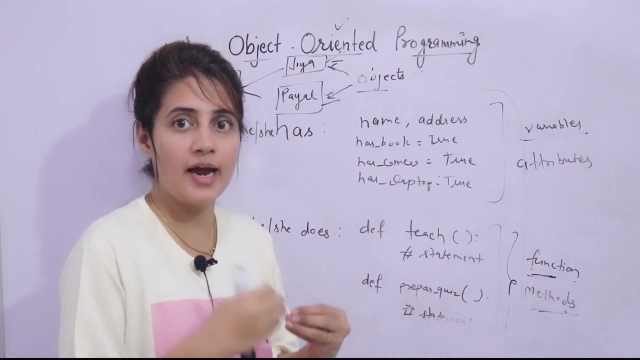 instructor was class, So it was just a blueprint to create objects, right? So we know like object oriented programming is used to model real world problems, real world objects, right? So every object is having some information and will do something. like I am an object, So I will have some information. 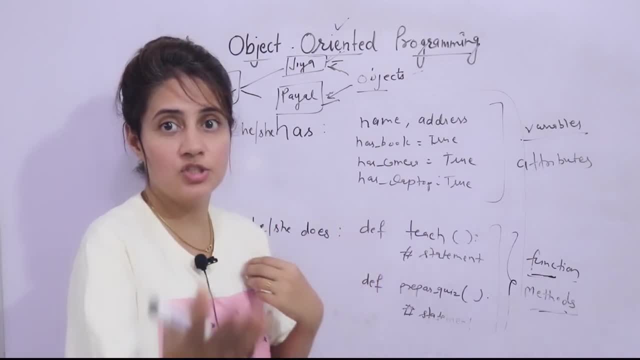 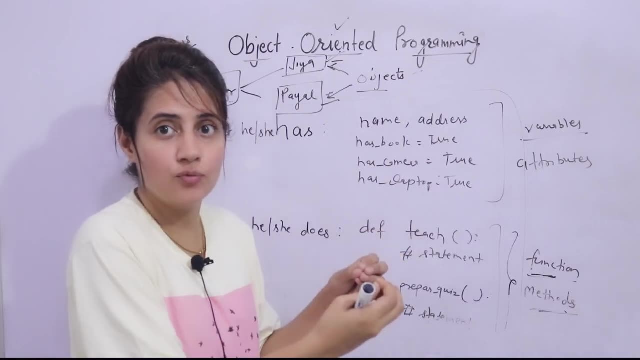 like name, phone number, address and I will do something. Maybe I am teaching right. So what an object have that we can model with the help of attributes and, or you can say variables and what I do. or what an object do that we can model with the help of functions or methods in programming. 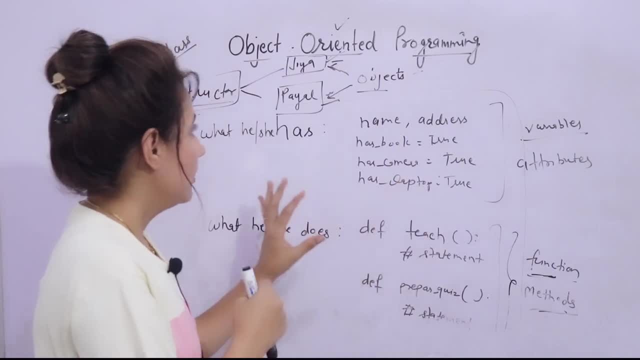 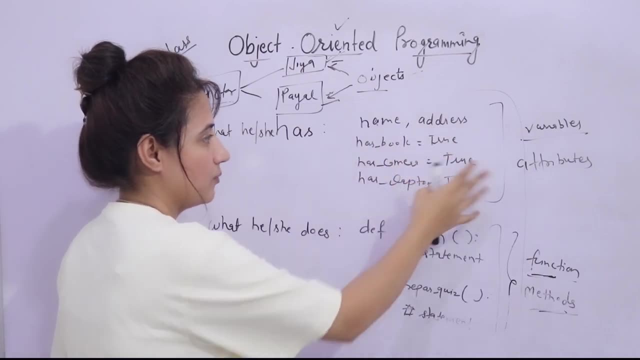 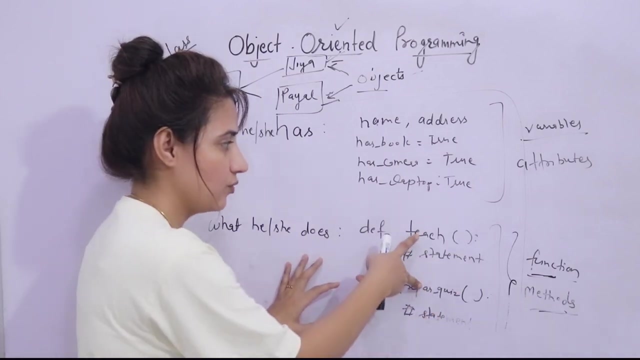 using OOP approach, right Here, like instructor, is having this thing, this information name address, and has book, has camera, has laptop and all and what the instructor will do: teach and prepare quiz. So these are methods or functions. See, we don't call these simple variables and functions. 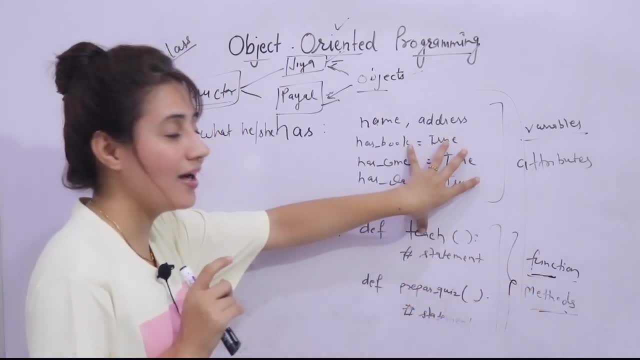 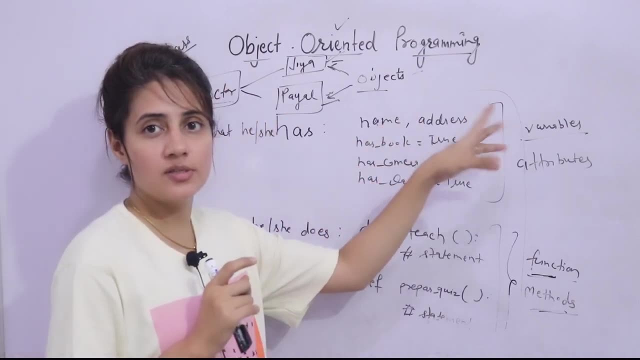 We call these attributes and methods. Why So? because these are associated. these are attached with the instructor. Like name is equal to Jenny address. I have some address, So these name and address are attached to me. These are not free floating variables. 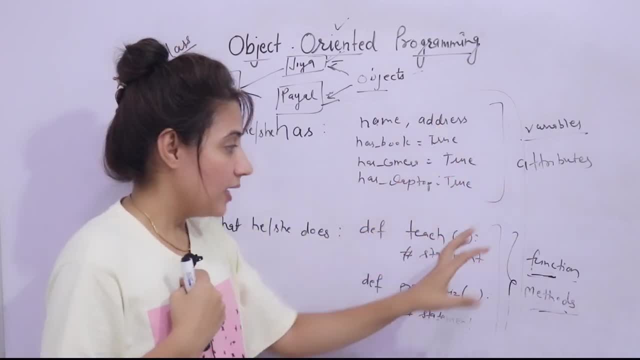 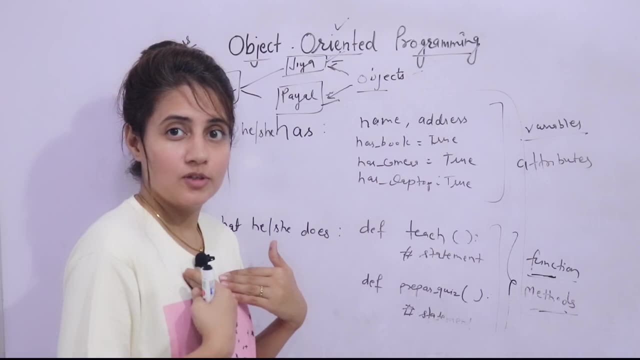 So these are attributes. That is why we call these attributes and the functions. like I teach, I prepare quiz. These are also attached to me if I am an object right, So that is why they are known as methods, not just simple functions that are free floating in your program. 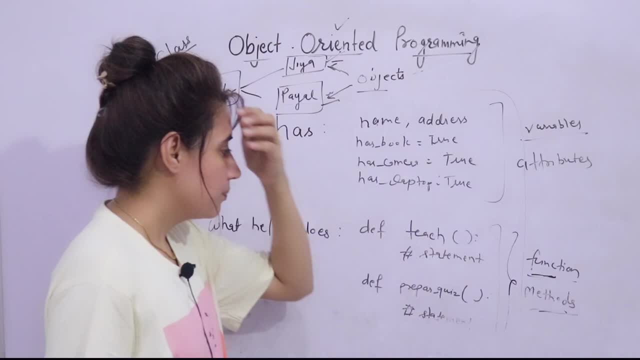 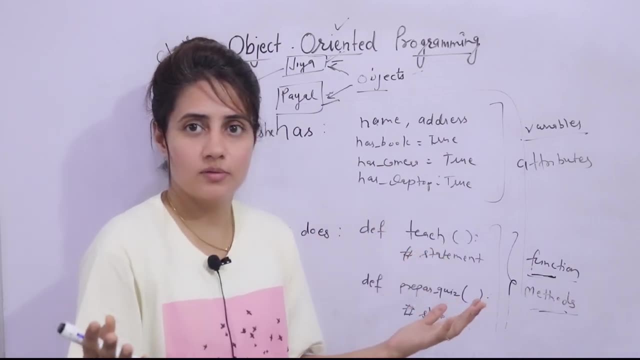 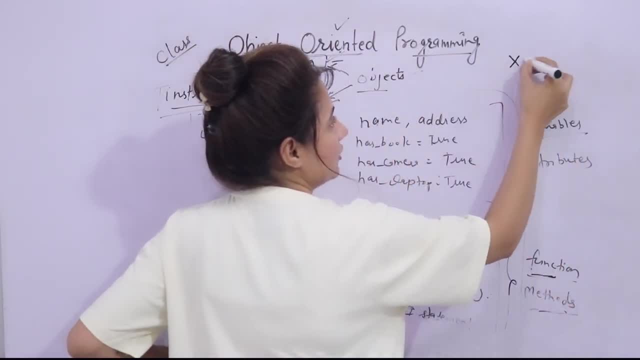 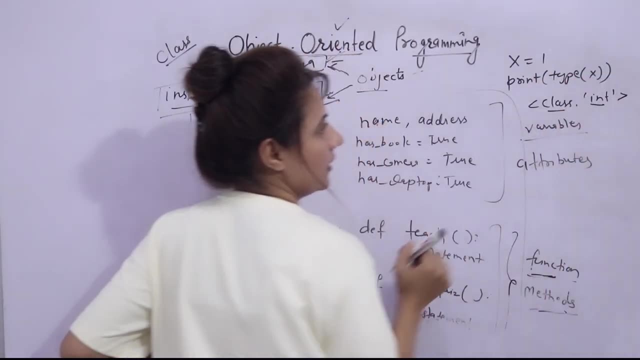 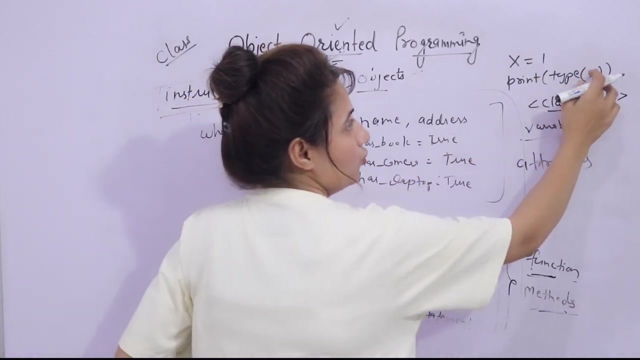 know I have given you one example also. simply, if I write x is equal to one and if I print type of this x, then what you will get Class int. So this x is an object of class int. The class has inbuilt class. if I want to find out like x in x, I'm having hello. So this is a. 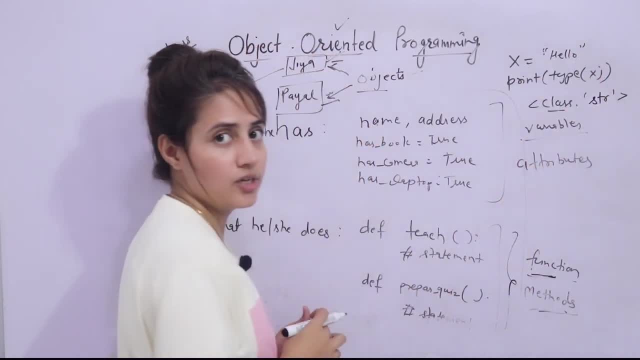 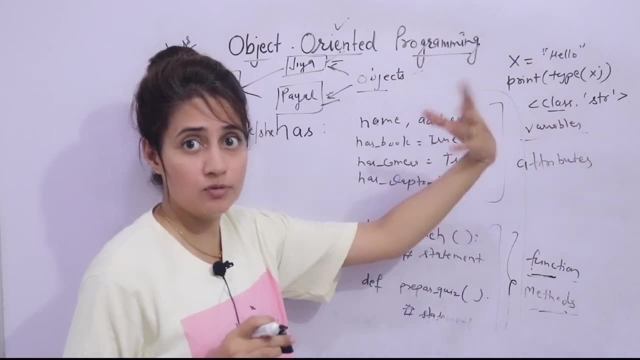 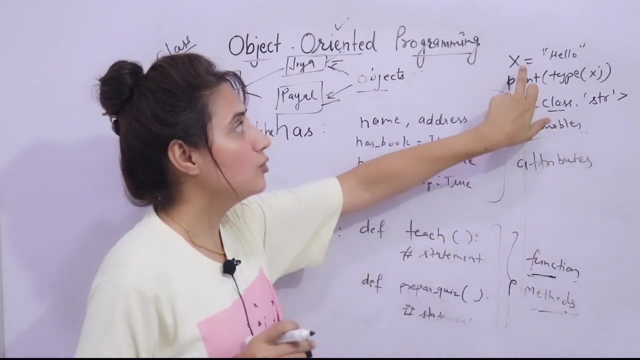 string. So at this time it will give class as str. So this is string. this hello. this x is an object, str, same with function. In the previous video I have shown you this thing practically right. So we have inbuilt classes in Python and we use the object. So objects are more important. 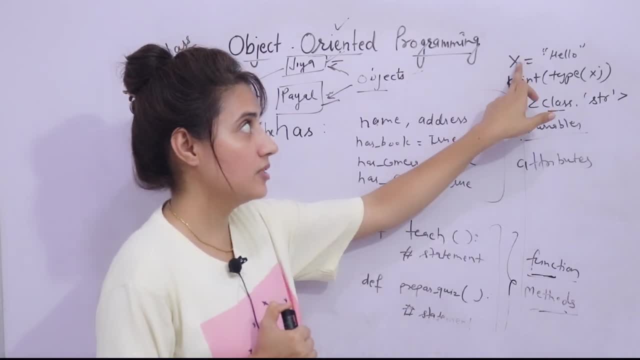 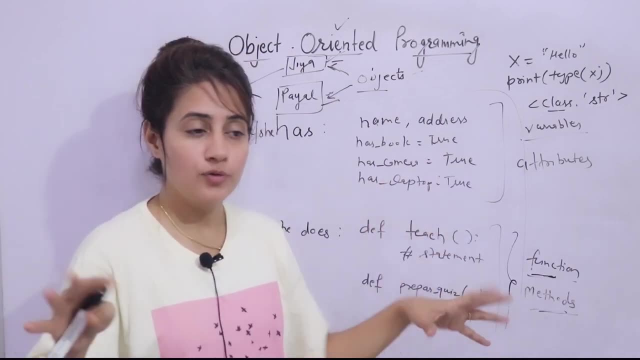 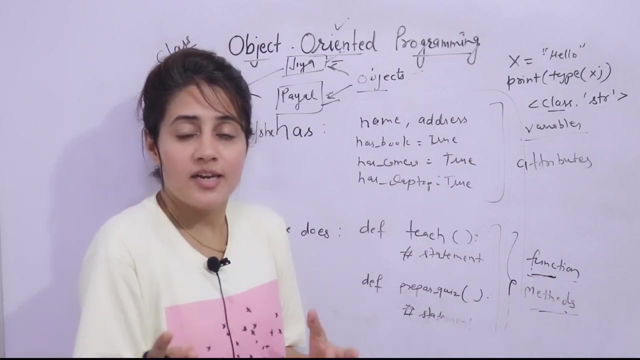 Everything we do with the help of objects: right, Because this x is an object, x1, this is an object. If you create a function, that is also an object, right. So objects are very important. We do everything with the help of objects in our Python, Python programming- right, Then if objects are, 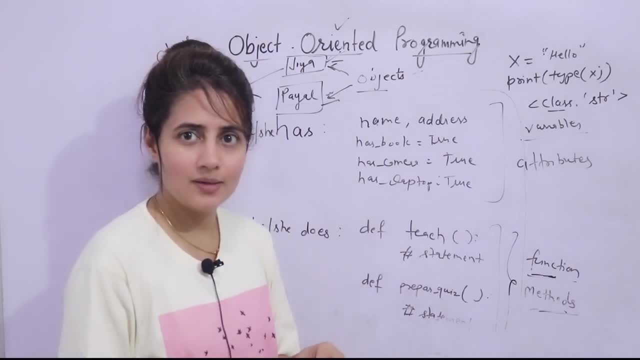 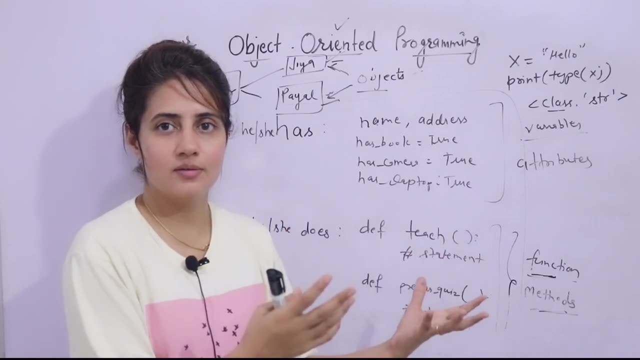 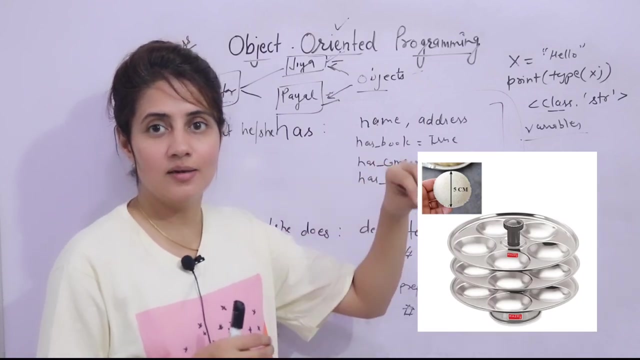 important then, why we need classes, right? Let's take, let's understand this thing with the help of this example. See, suppose, like you have an idli maker, right? So this is an idli maker and you put that batter or that stuff here in this idli maker and your idli will be ready in next. 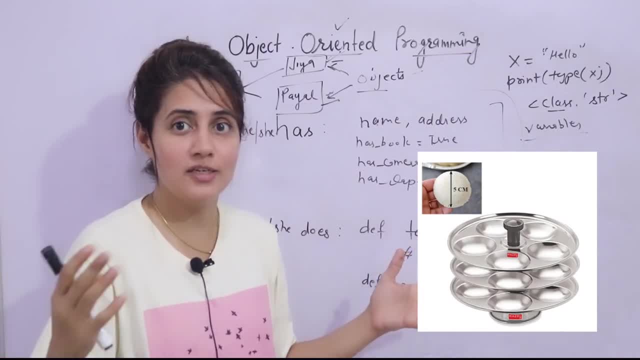 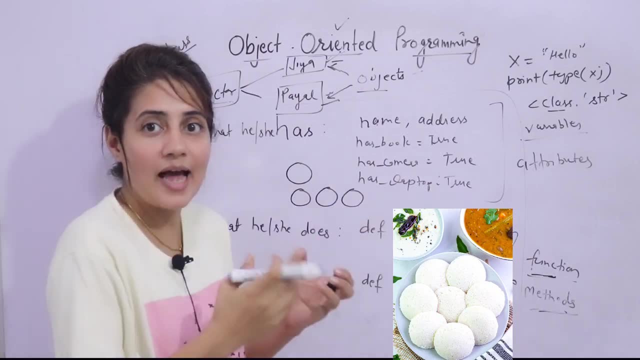 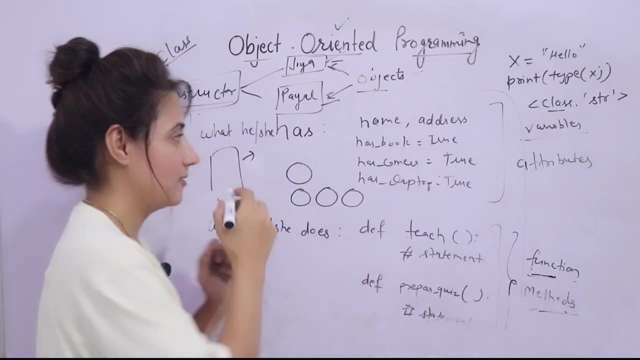 maybe I don't know the recipe- Or maybe 10 to 15 minutes, within 10 to 15 minutes, right? So the idli you are having- these are actual objects- and the idli maker- what you have, that is just a design. 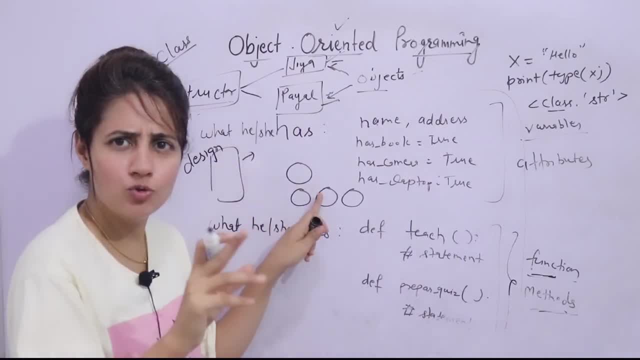 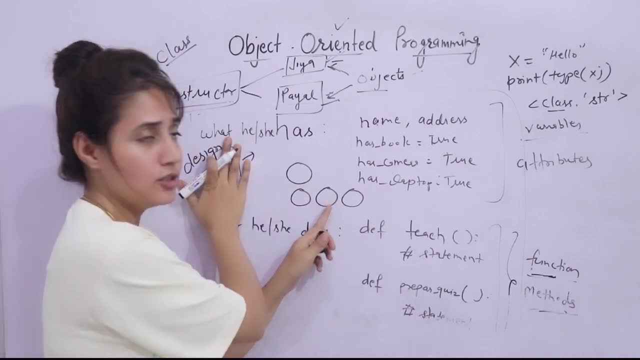 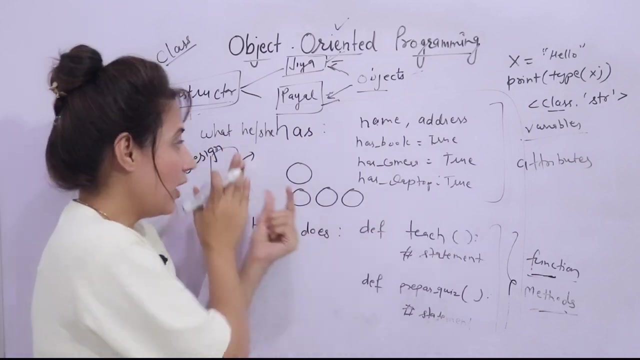 to make to prepare idlis right, And if you don't have this design, then I think it would not be easy for you to prepare idli. Maybe you can prepare with the help of some other method, I don't know. But if you have this idli maker, then it is very easy for you guys to 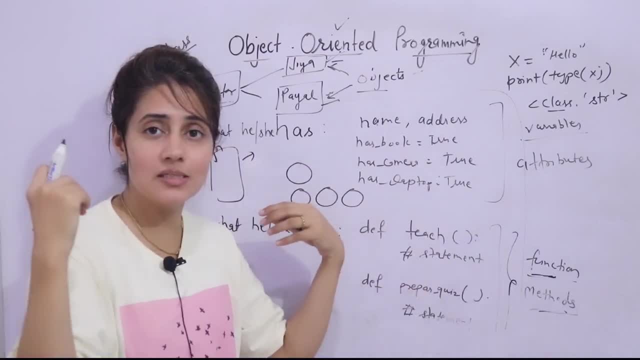 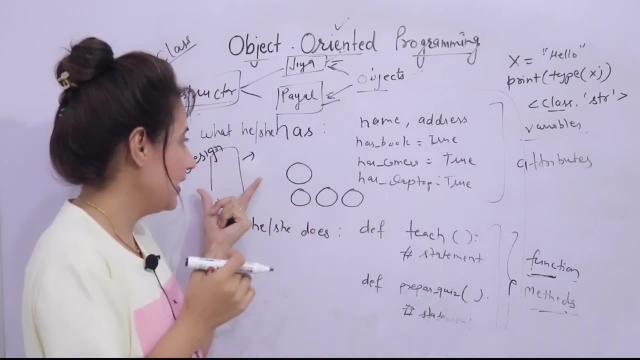 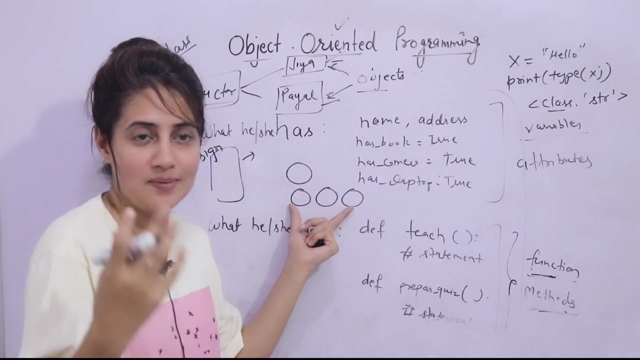 prepare many idlis just in just you know few, maybe hours or few minutes, right? So this idli maker is going to make your thing, to make your- you know- process of making idlis very smooth and simple and quick, right? So it is a design. Same if you relate this thing with the help of example. 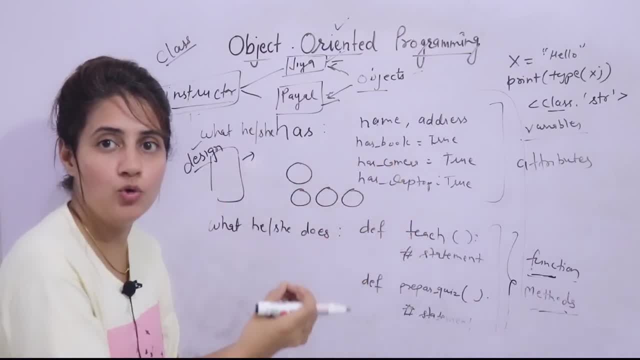 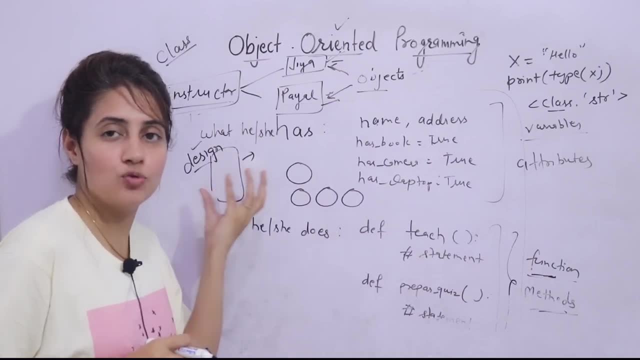 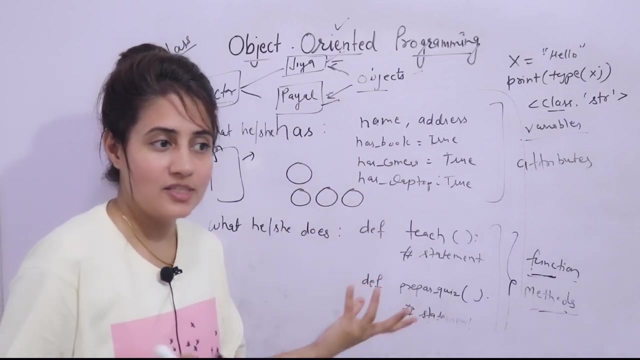 with the help of example. So class is just a design or blueprint. So, obviously, to create object, to create idli, we need idli maker, So we need a class. to create object, we need a class. That is why classes are important. Same like if you have any car, like maybe: 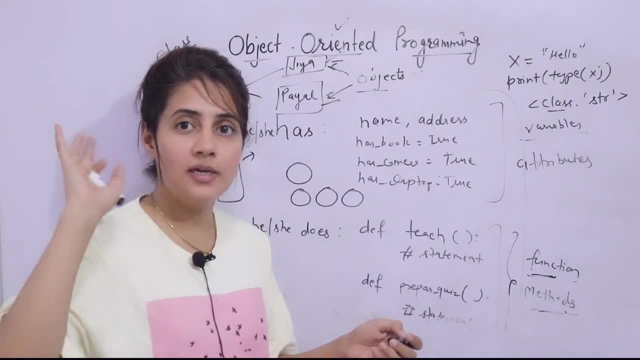 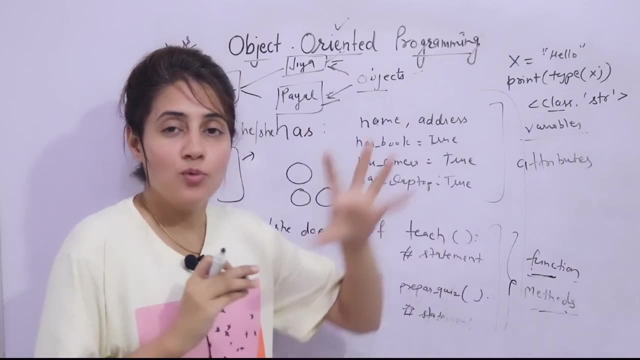 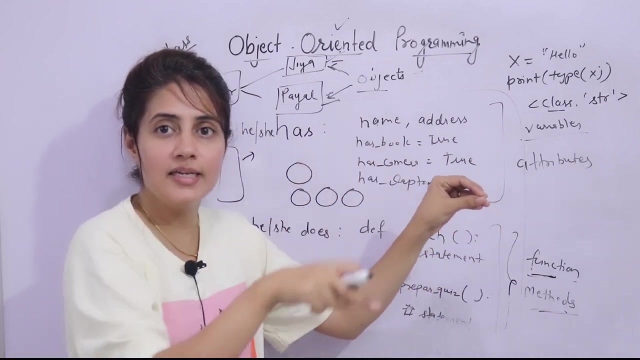 Creta. So there are, let's suppose, 1 million Creta in India, right? I don't know the number, but I'm just supposing the thing. So there is a model there, there is a prototype, there is a design of that car Creta, and using that design, they are creating multiple Cretas in 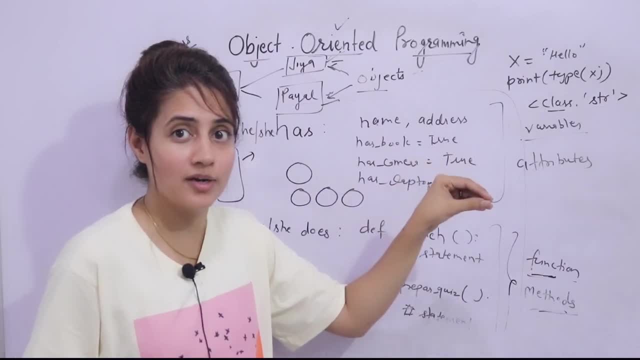 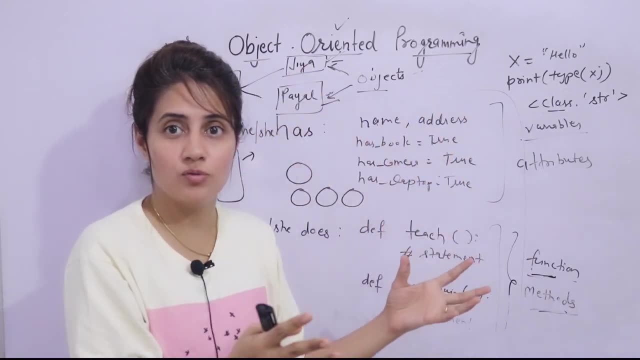 less amount of time. So that design is important, that blueprint is important. Same like third example we can take like a map of a house or a sketch of a house. right Using that sketch we can create house, houses, many houses. 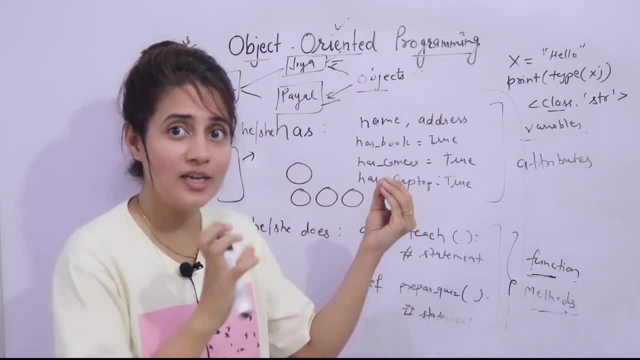 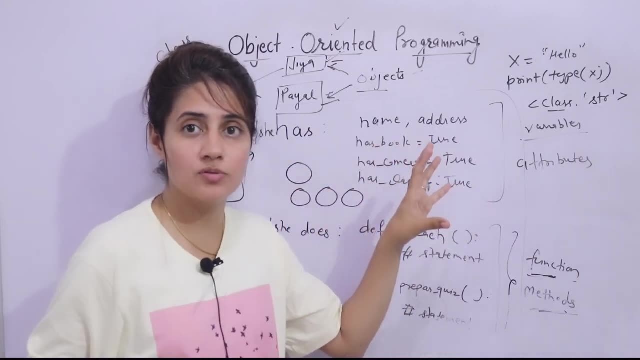 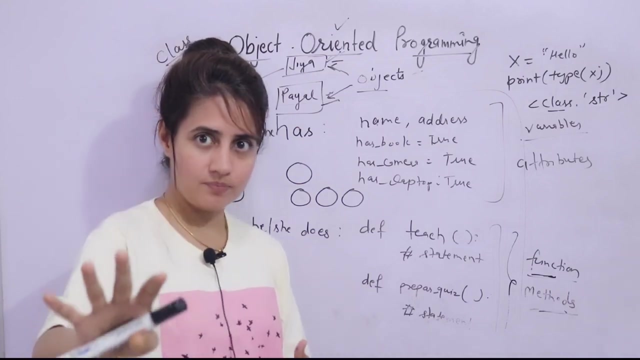 So that house you create an object, the real thing that is an object, and that map is just a class or a blueprint. But using that blueprint you can create multiple house, multiple houses, many houses, right? And if you don't have that map, then definitely you can build, or 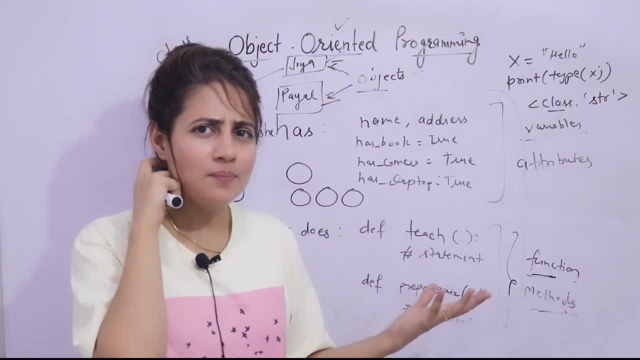 you can construct a house, But if you have map, then it would be easy and, you know, simple to build a house, to construct a house Because there are many people who are building houses and there are many people working there and one who know like what is the map, exact planning? 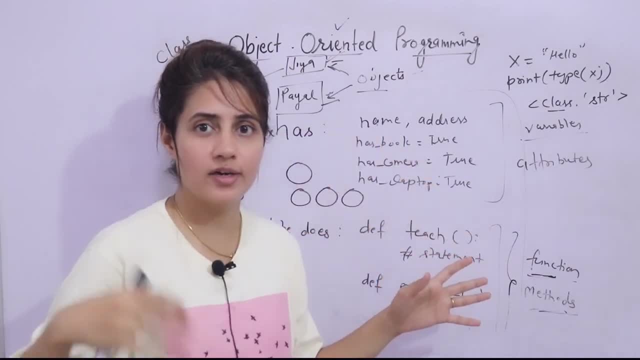 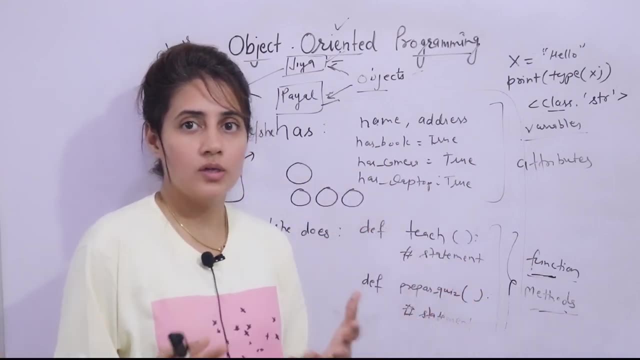 like what to do next. then he or she can easily guide the contractor or anyone. He or she can easily guide to the members what to do next. If you don't have map then it would be not that much easy to communicate, So relationship would be tough right. 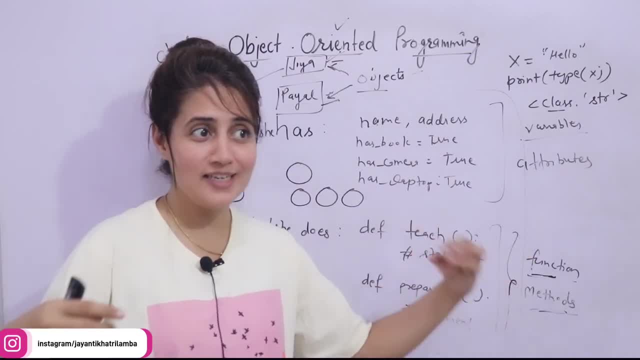 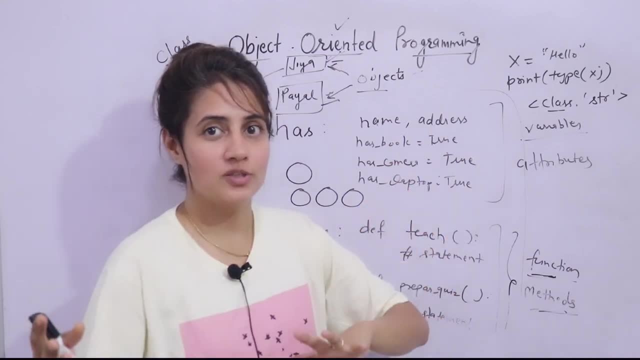 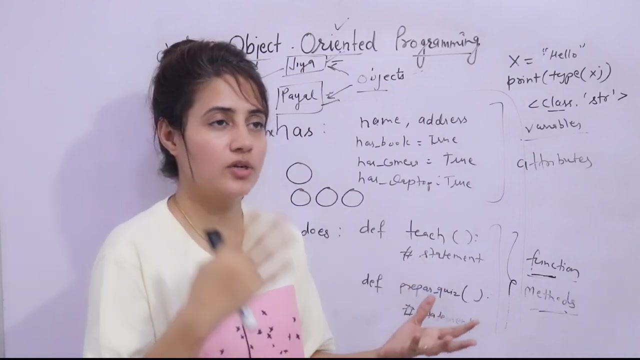 So now I hope you got the idea of class and object and why we need class. Class is also important, right? So we can say this class is just a blueprint or a design to create object, An object, or you can say instance. we can also say: Object is an instance of that class or instance of 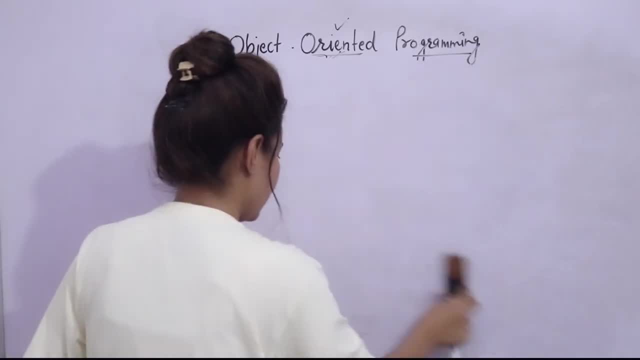 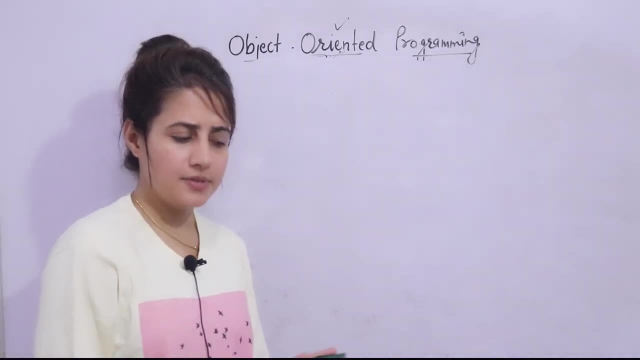 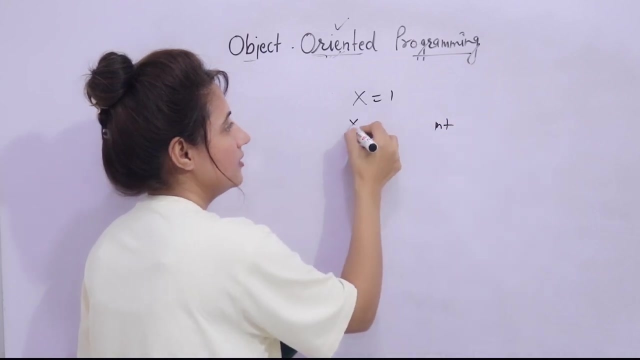 a class, right. Or we can say: class is a user defined data type, user defined type. Why I am saying so? Because, see, when you take x is equal to 1, the type of x is int. When I say x is equal to hello. 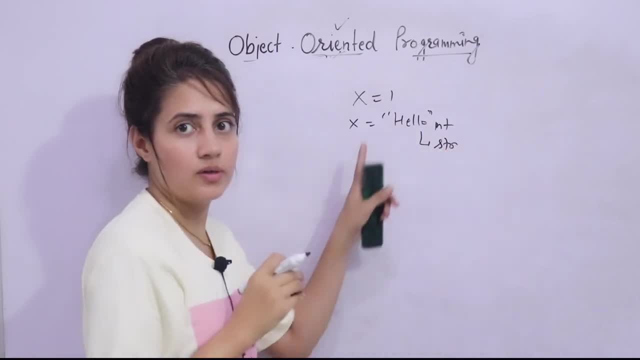 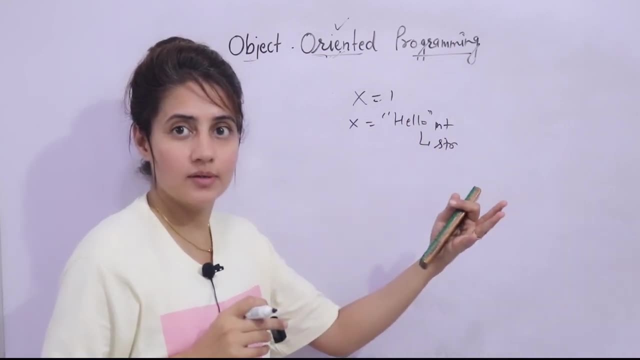 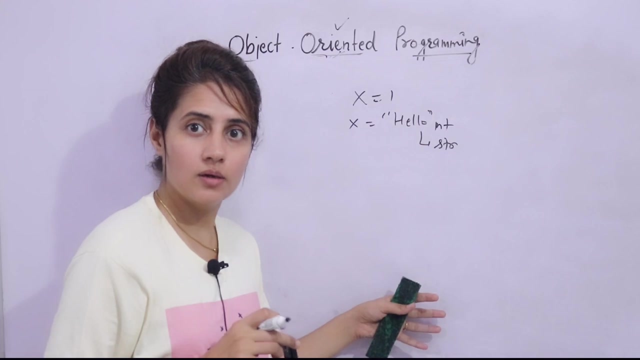 Then the type of this is: it is of class str, it is of class int. So these classes are inbuilt classes right, Like int, str or many classes. we have Boolean also we have float double right. So if you want a variable, something like this: so 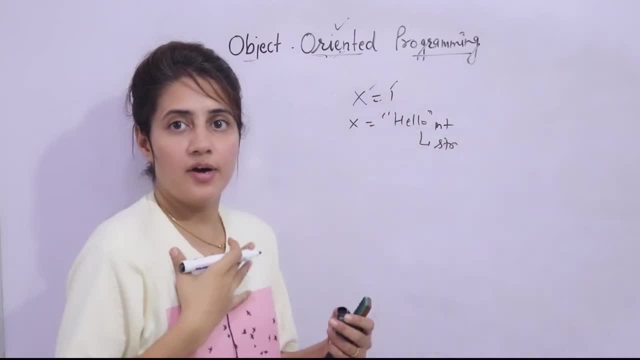 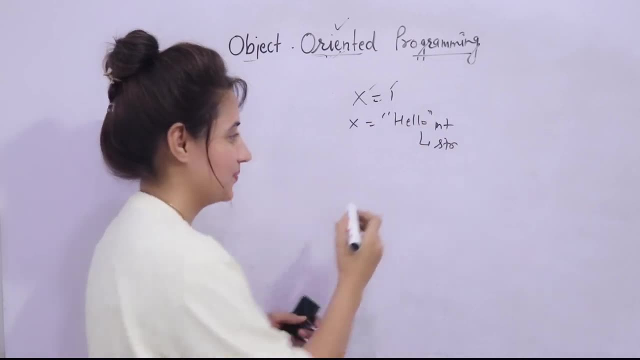 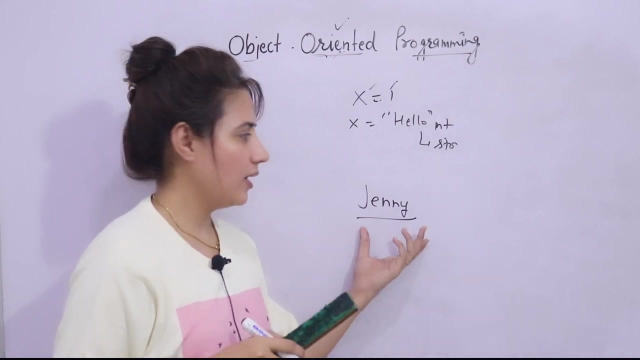 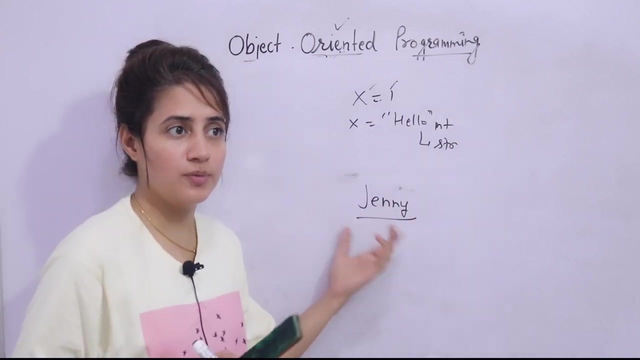 the type of this is already defined like int, But if I want like a, I want like a type of class. If, like Jenny, an instructor, so this would be of like this is not any type, like. I am not providing it as a string, but Jenny is like an object, it is having some information. 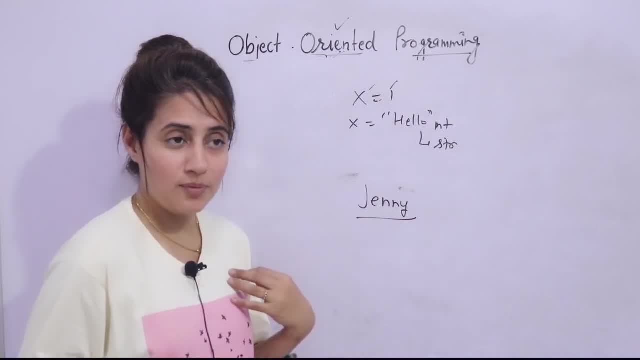 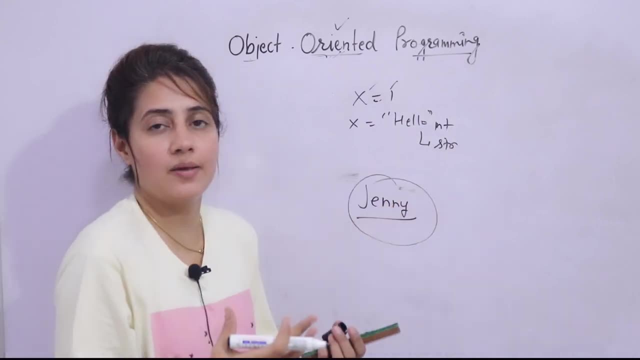 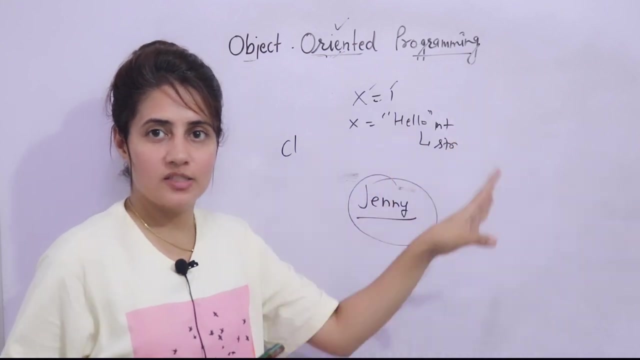 like me as an actual person, real person, some information, I am having, some task I do right. So for this we have to define our own type right, So that we can define with the help of, like class keyword and whatever class name you. 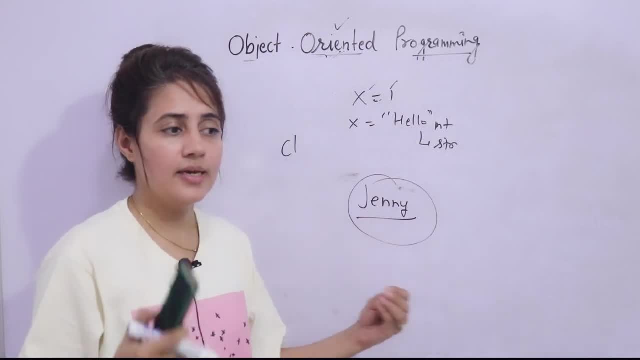 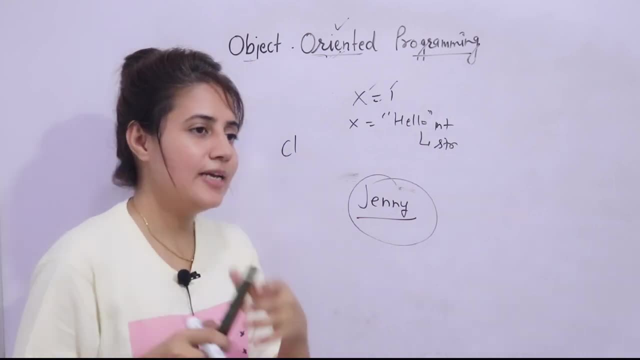 give right. So class. simply we can say it is a user-defined data type also. okay, This thing, class is a user-defined data type, that you will get it at the end of this video. don't worry if you are not getting this right. 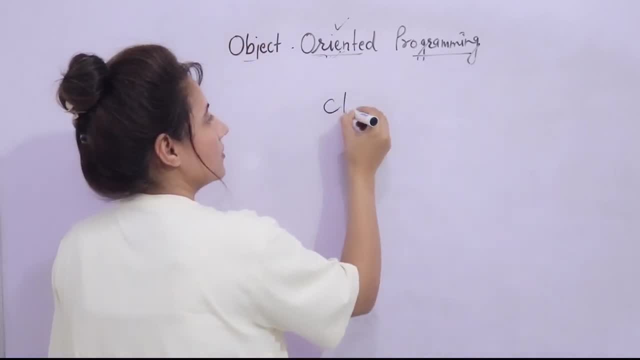 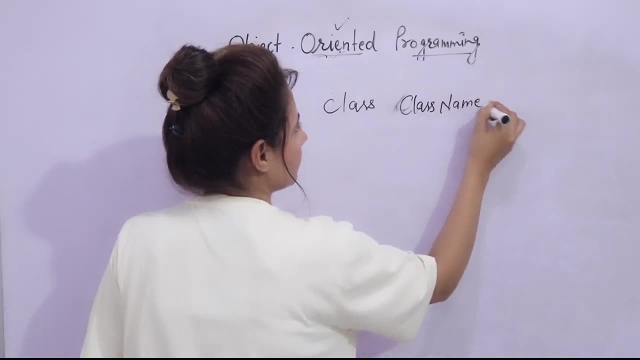 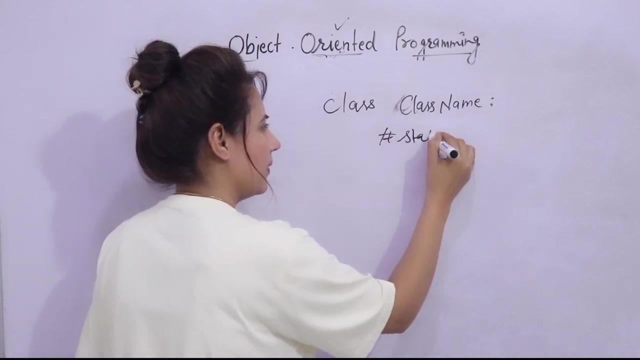 So syntax of creating a class, how to create your own class, Just class keyword and class name, right And column, and here obviously the data, what you want to write here, the attribute and the methods, and that also we will see right. 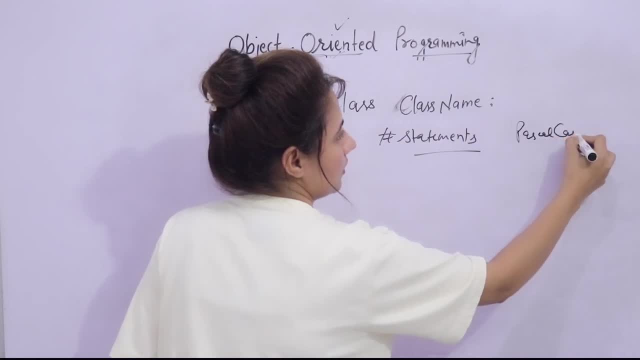 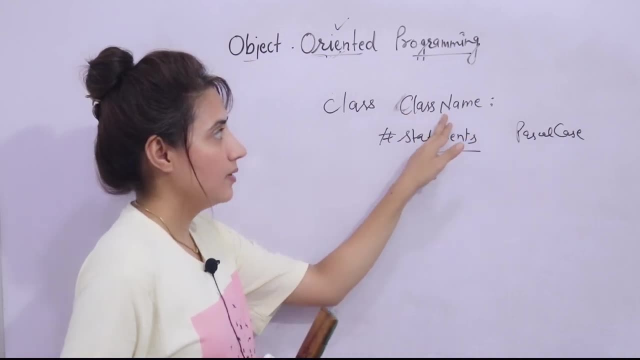 The class name is. in Pascal case it means the. you know, first letter of each word is capital letter, like class. the name N, like our name, Jayanti Khatri, so J is capital, K is capital, like this, So we use this language. 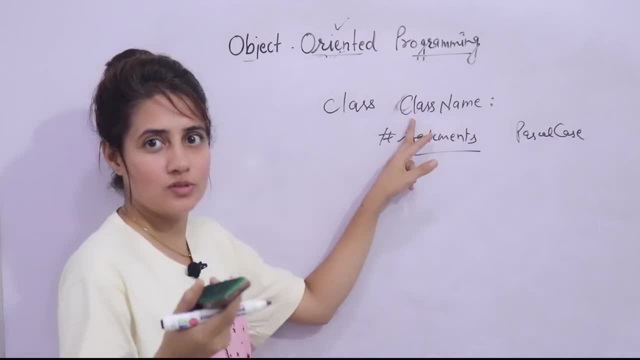 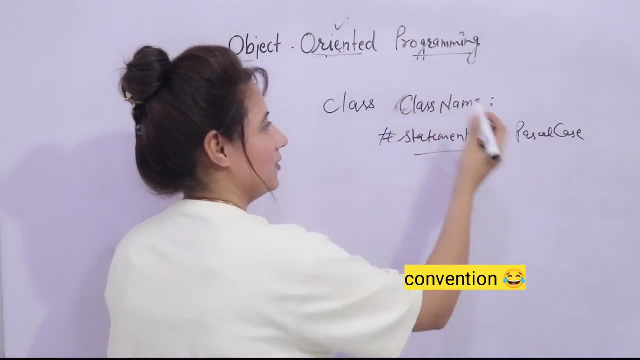 Okay. Okay, You can say the, but I should say this: I'm not. I'm not getting the exact word, it's okay. So this is: you can say some kind of rule you have to use, like Pascal case, to write. 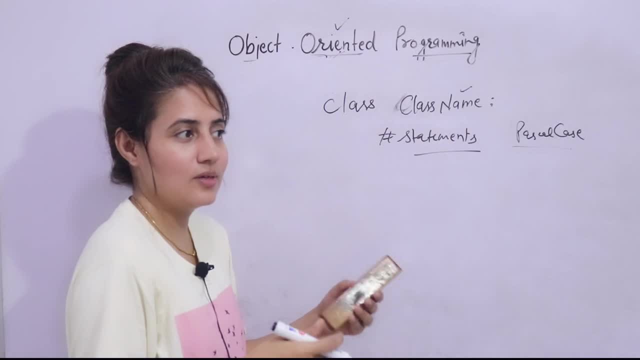 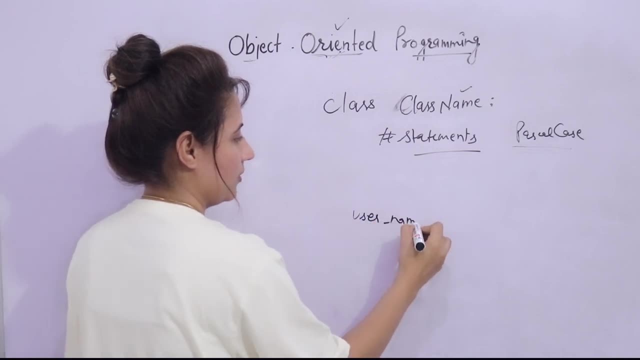 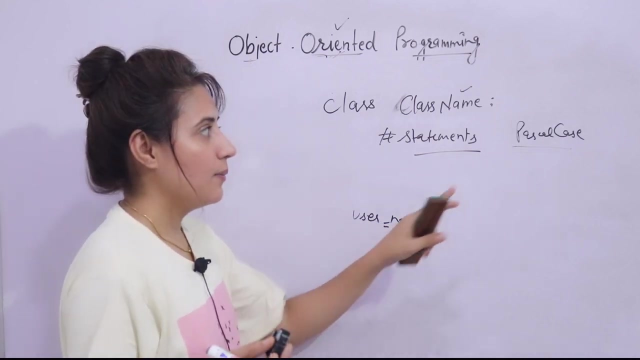 down a class name, like for for creating variable name. we simply use like underscore, like maybe, I don't know, like user underscore name. if a variable, then we use underscore. This is a snake case, right, Camel case is also there. 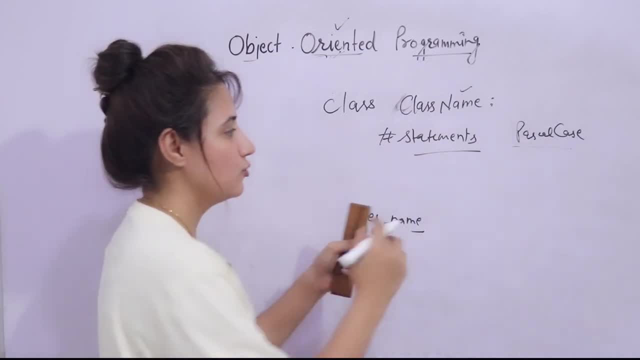 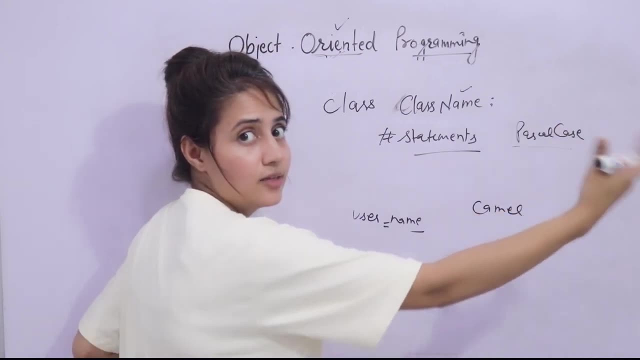 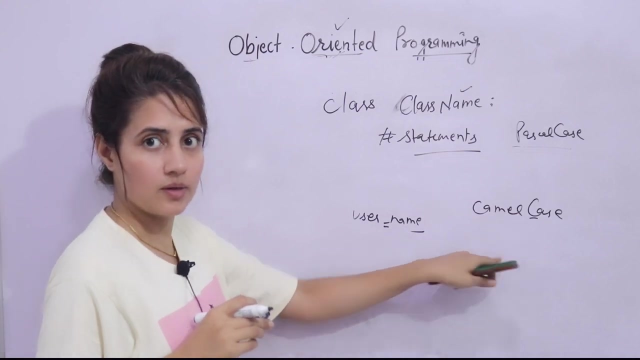 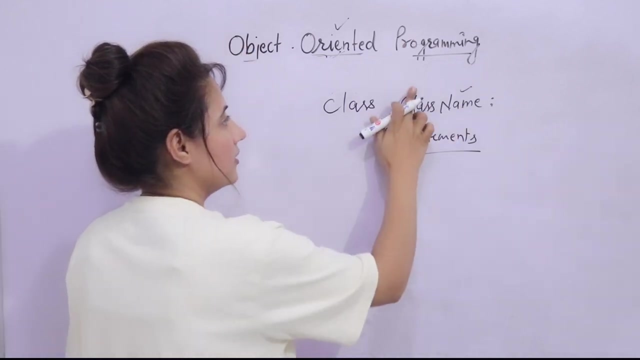 In camel case. So first, first is what First is. letter is small and for each other words, the first letter is capital. This is the only difference between Pascal and camel case, right? So this is how you write class, class name, or if you write like something like this: 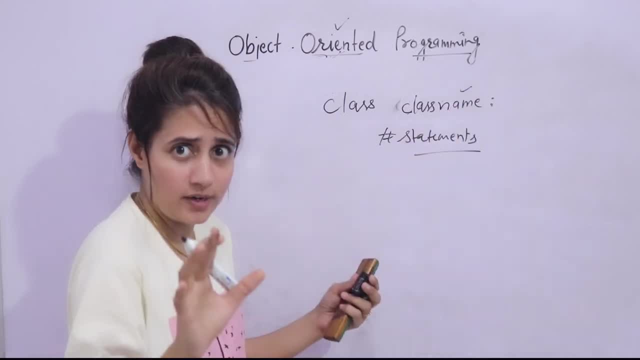 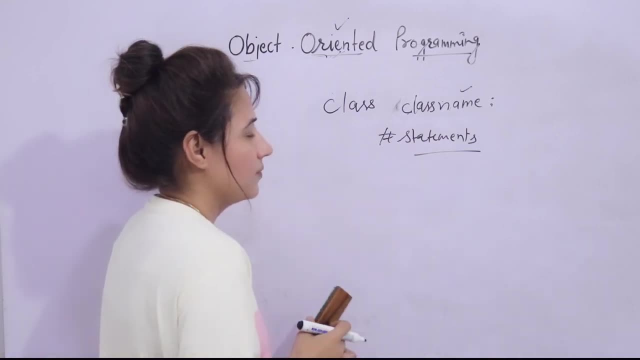 first is small, this is also small, that also will be fine, It will not give you any error. Okay, But that is some kind of you know rule, or you can say this kind of thing right, Just to differentiate between a class name, a function name or a variable name, something. 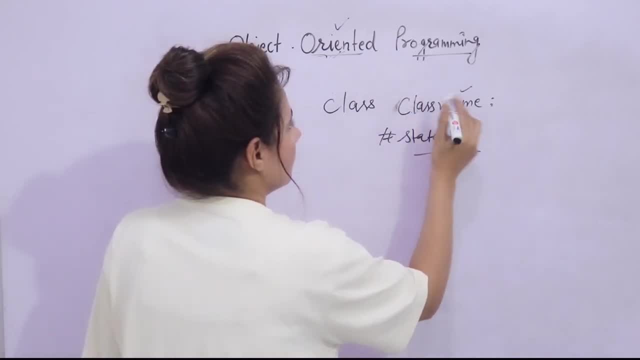 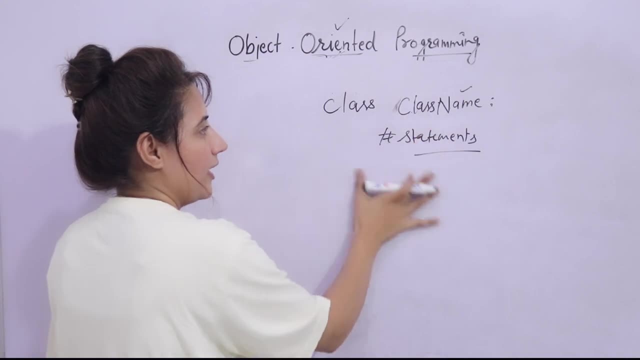 like this right? So like this: we write class name. fine, This is the syntax, simple, And here you will write whatever you want to like: attribute methods and all that also. we'll see Now how to create object If from this. if suppose class name is instructor. 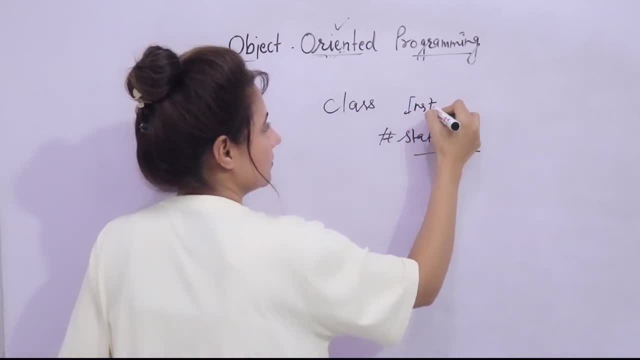 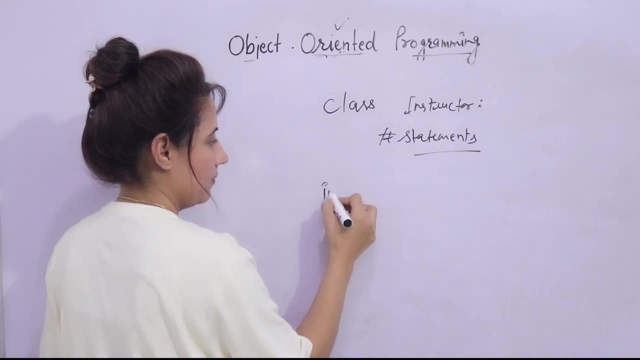 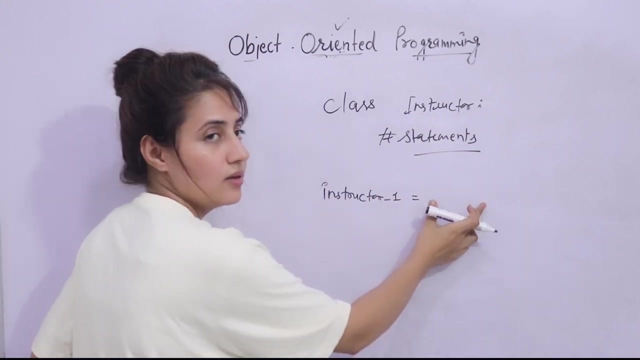 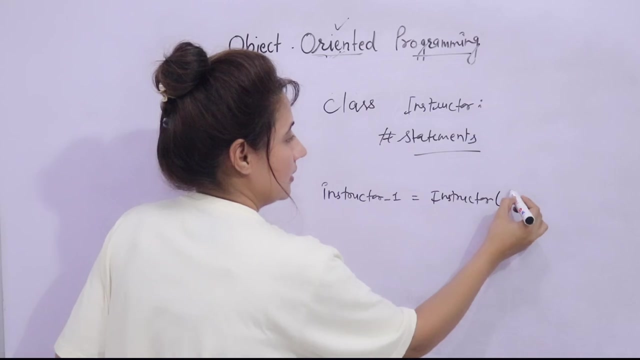 Okay, Okay, Okay. If I want to create object of this class, then maybe I am like writing instructor underscore one is equal to just the object name, then class name. class name is instructor. But this is not it, This. you need to pass the these brackets down, brackets. 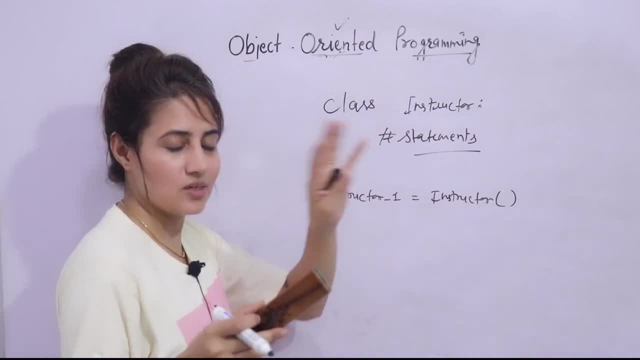 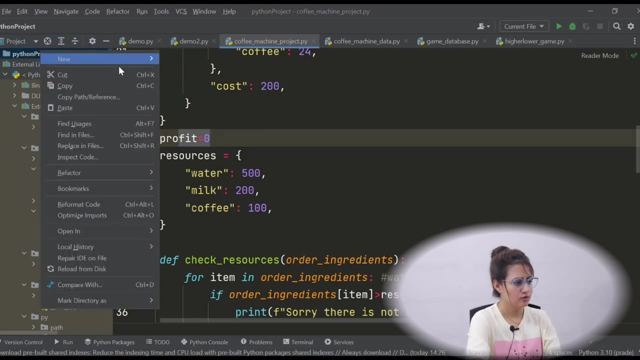 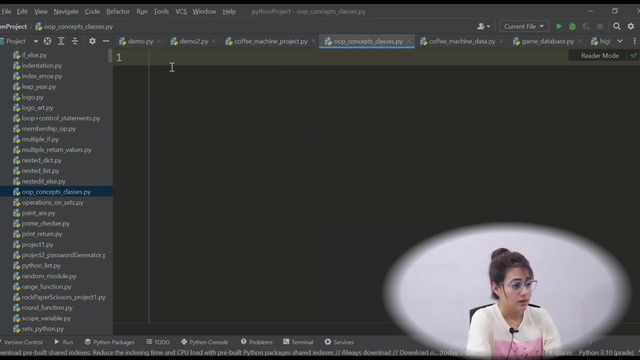 So this is somewhat like constructor. Now, what is constructor? that also we'll see. But this is simple syntax of creating an object. Let's see this practically Okay. So let's create a new file: OOP, concepts, classes, dot, py. So how to create your own class? just class keyword and class name. 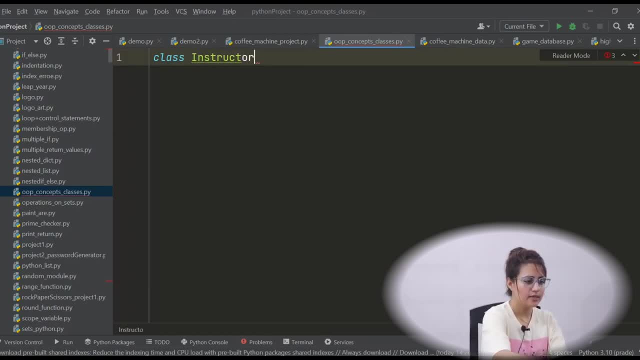 So I am creating a class instructor. Okay, Okay, So I am creating a class instructor. So sorry, Pascal Pascal, cases first is capital, and if the next, if you want to write on like information, I-N-F-O info, then I would be again capital. 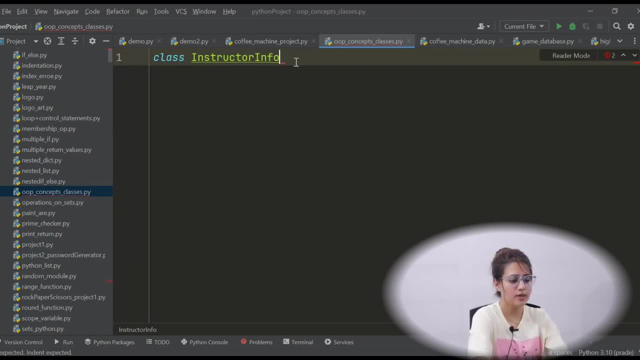 So this is Pascal case. Every letter of the word would be capital, So just instructor and then column. Right Now, okay, I'm not passing anything in class. no attribute, no method. So maybe you think this is an empty class. 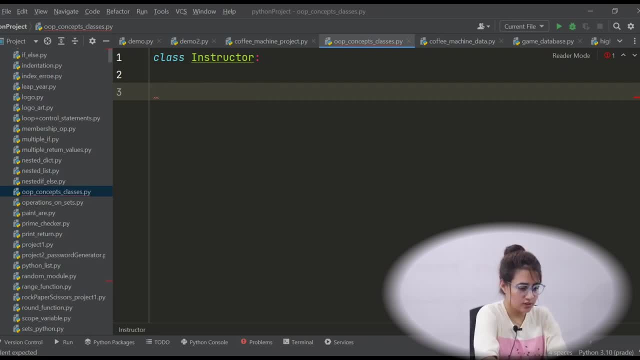 Right, And I want to create object of this class, So instructor one. the name of the object is instructor one, and then equal to the name of the class: instructor and just these brackets. But see now, can you see this red line here? 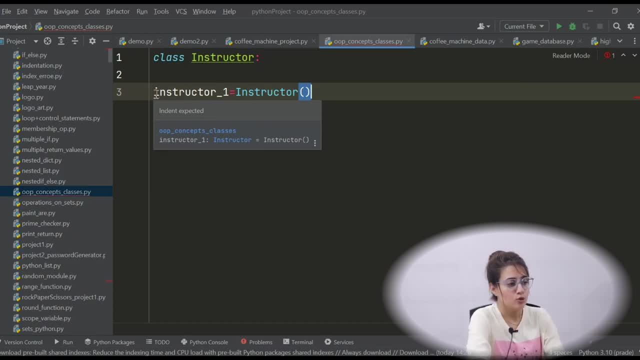 So this is an error. like this indent expected. So same with function. I think you have seen, if you create function, then you cannot, you know, leave that function empty. You have to write on something, but I'm not, I don't want like I don't know how, what. 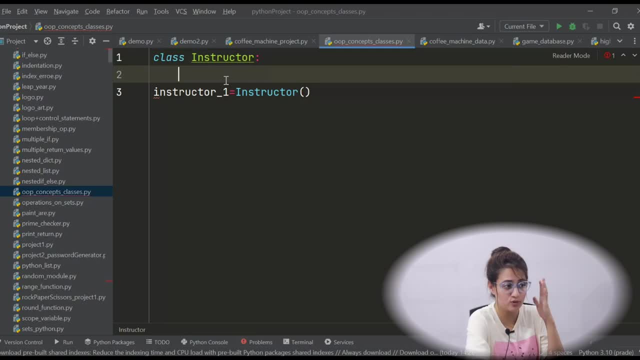 to write in this class right now. I don't know the syntax, how to write attribute and methods. So I have told you one statement we have: pass So that you can select. just write down here. pass, So maybe further I'll do something here, but write down. I don't know what to do here. 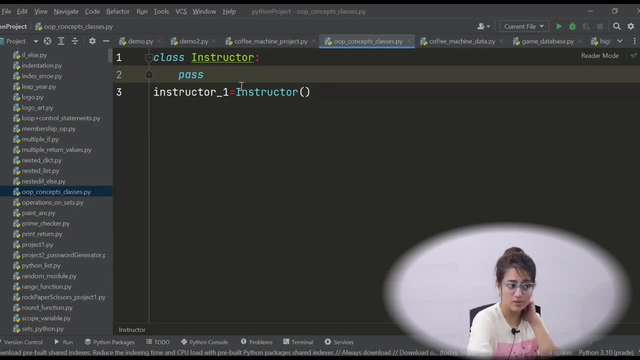 So just write down there, pass. So now see there is no error. Okay, Okay. So this is how you can create your class and this is how you can create an object. So if you run this, then there would be no error, but no output you will get. obviously. 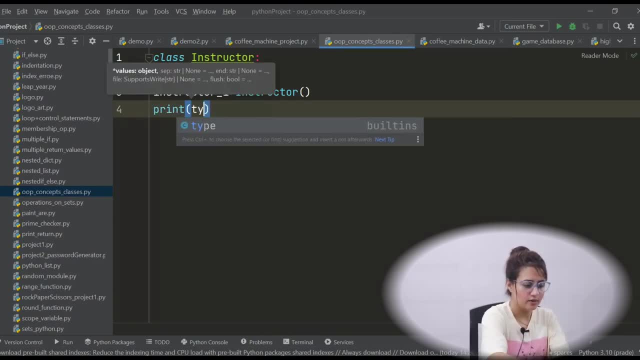 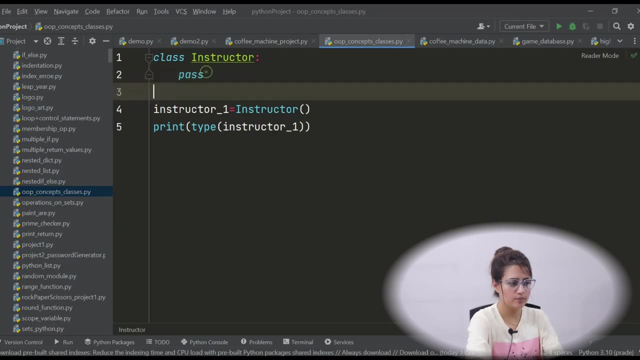 Now, if you want to find out the type of this object, type of the object: instructor one, because name of the object is instructor one right. This is the name of the object we have created. So what should be the type of this object? 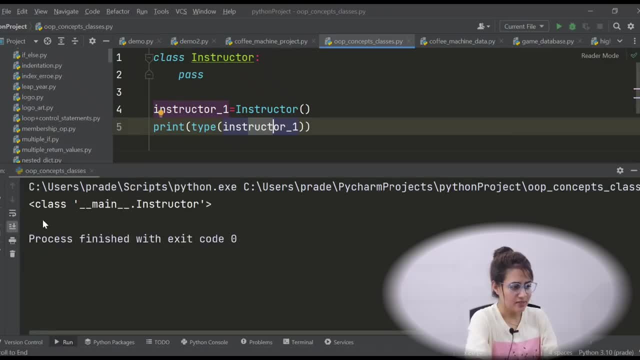 Let's run this. See, the type is class is just focus on the class. instructor- right, Although we have underscore, underscore, main underscore, underscore, So that this thing I'll be talking in later videos, right, But now you have to focus only on this name: instructor, right. 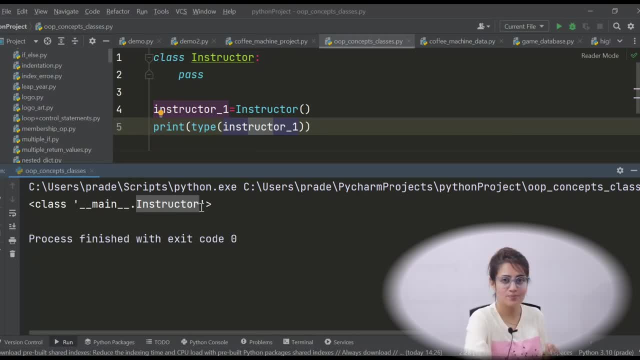 So now we have created our own type, our own data type. That is why I have told you that line like class, is a user defined data type as well. Okay, Now, as many object as we want we can create from this class, from this type. instructor. 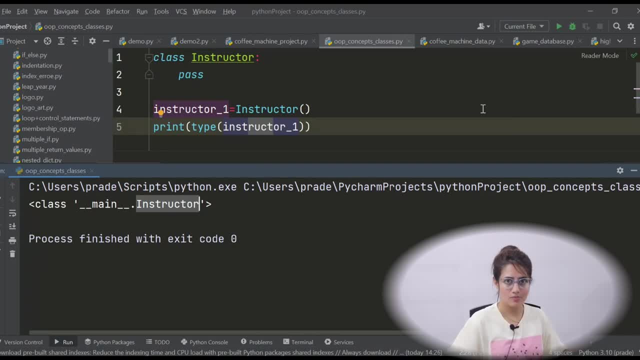 one, two, three or many objects, many instructors right, But all would be of this type: class instructor. So this is a user defined data type that actually acts as a blueprint to create objects right, And object is just an instance of a class right. 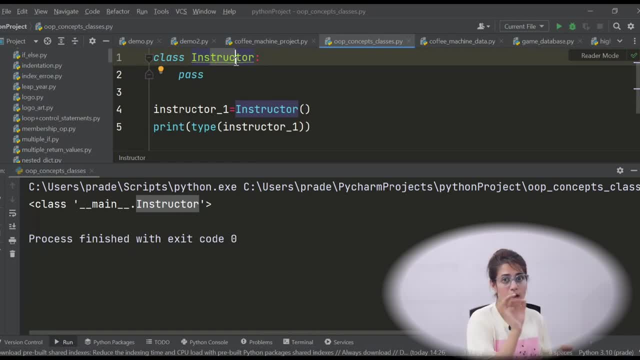 Now one assignment for you is you have to create a class and the class name would be car design, car design- This would be your class name. Okay, This would be the name of the class, right, And you have to create two object of that class right. 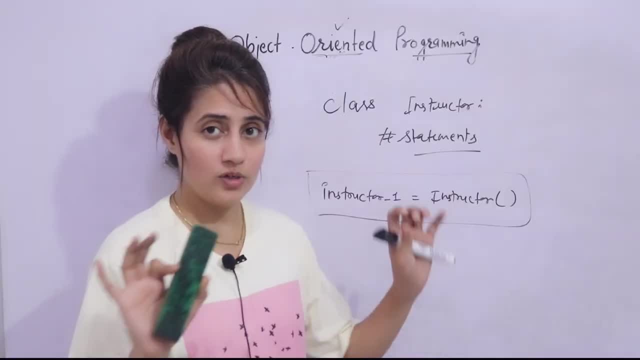 So this is your assignment. You can write on that thing in comment section. So now I hope you got what is a class, what is an object, what is object oriented programming, how to create your class, how to create an object right. 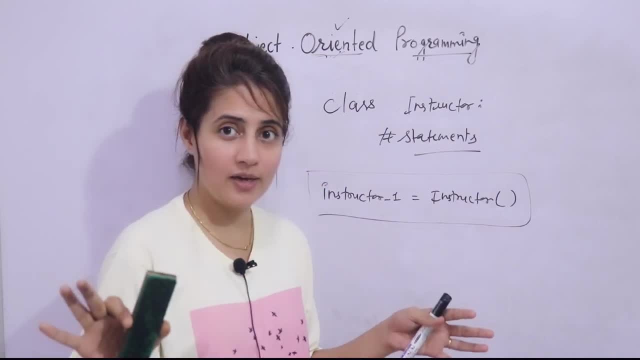 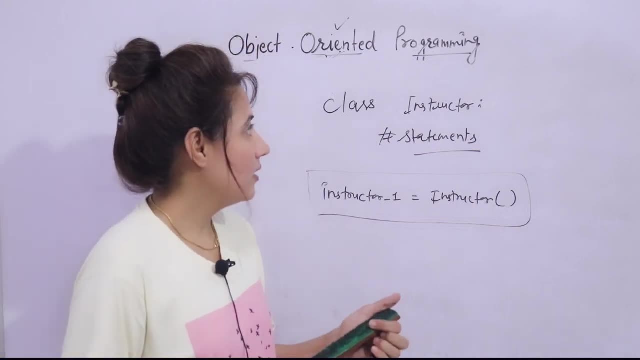 If you are not getting this, if you are still getting like 50%, then it's fine. You know, slowly you will get everything in later videos. right Now, in the next video, we'll see, like, how to add attribute to your class. 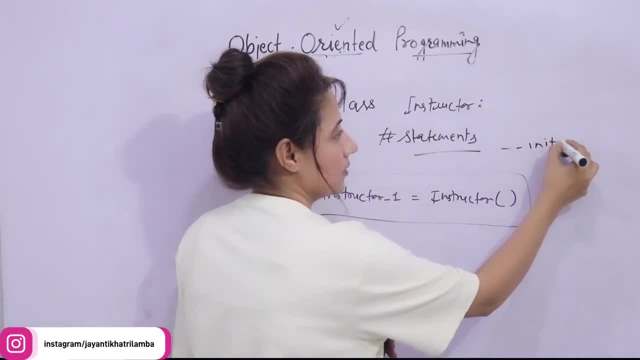 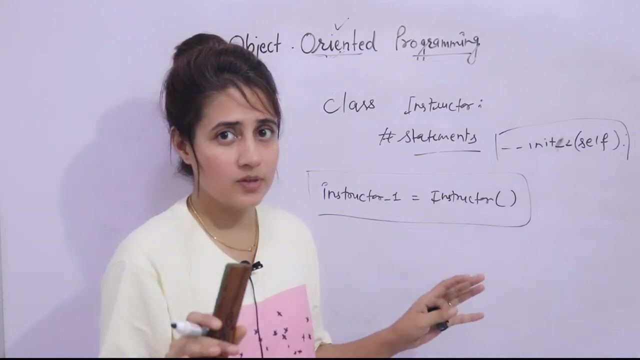 There is a method like init that also we will see in next video, like underscore, underscore, init, underscore, underscore, then in bracket cell. So what is this method that also we'll see in next video? What is constructor, This kind of concept, right? So I'll see you now in the next video. till then, bye, take care.